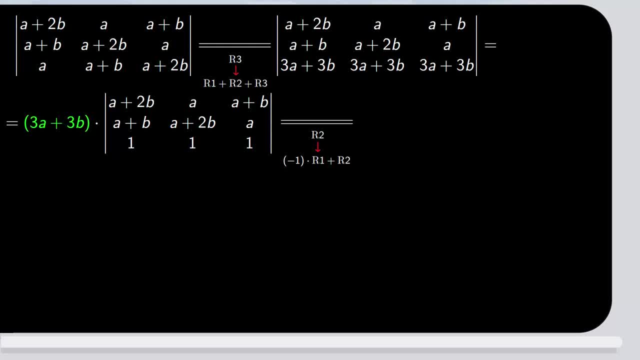 This is what we're left with. Instead of 3a plus 3b, we take out a common factor of 3 and write 3 times a plus b. This is times the determinant. We copy the first and third row and replace the second row with the second row minus the first row. 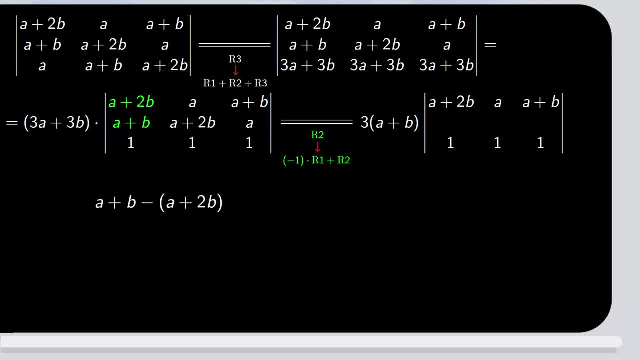 We have a plus b minus a plus 2b is minus b, a plus 2b minus a is 2b, And a minus a plus b is minus b. Just be careful with the signs. Now we have a common factor in the elements of the second row, namely b. 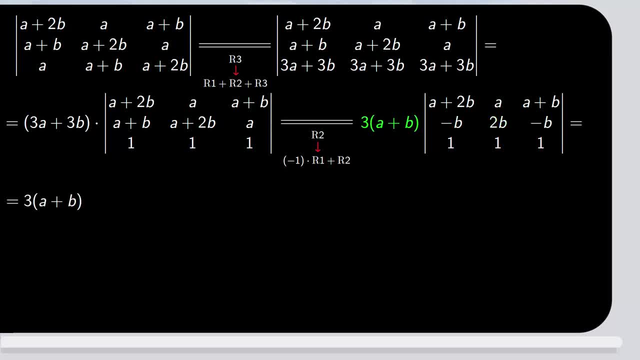 It comes out of the determinant. so we have 3 times a plus b times b and now the determinant. We copy the first and third rows and in the second row, after taking out b, we have minus 1, 2, minus 1.. 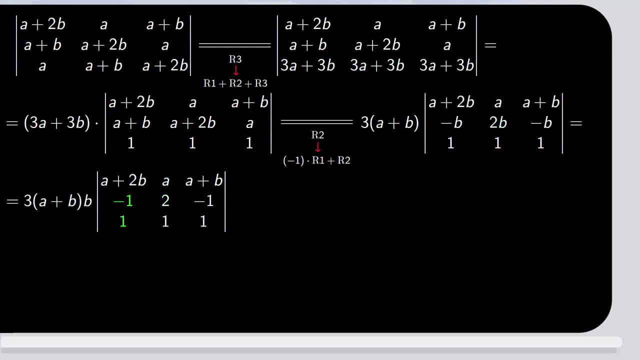 Notice that if we add the second and third rows here and here, we get 0.. So for the third row we can substitute the second row plus the third. We have 3 times a plus b times, b times the determinant. 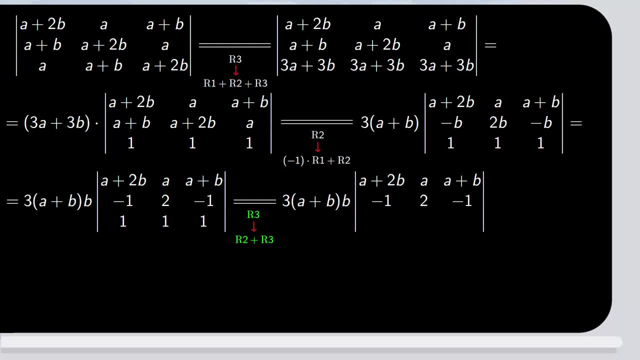 We copy the first and second row and instead of the third row we have the second. add the third row. Minus 1 plus 1 is 0.. 2 plus 1 is 3.. And minus 1 plus 1 is 0.. 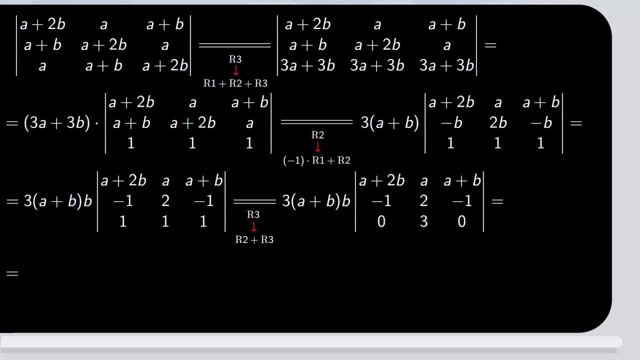 Now we can easily develop the determinant by the third row. We copy 3 times a plus b times b. In the third row we only have this non-null element. The determinant is 3, and for its adjoint it's in the third row and second column. 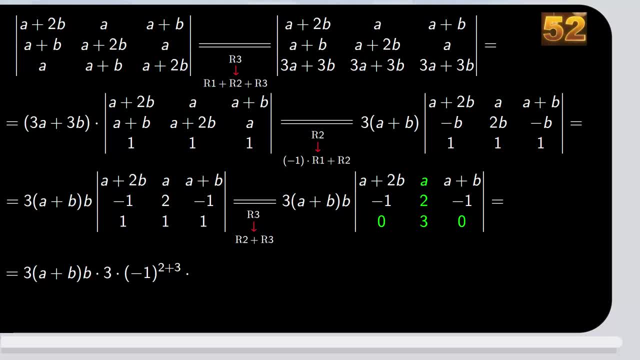 Minus 1 raised to 2 plus 3.. This is multiplied by the determinant that results from eliminating its row and column. And there it is To finish off. minus 1 raised to 2 plus 3 is minus 1 raised to 5, which is minus 1.. 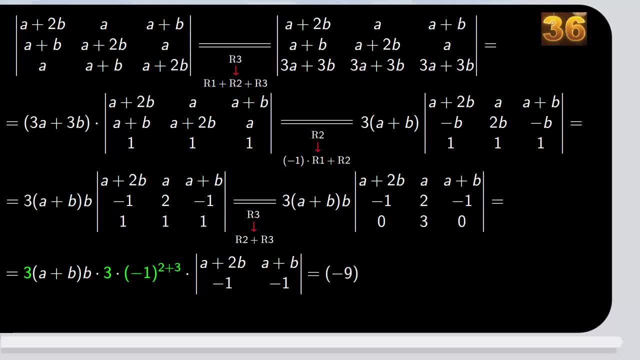 Multiplied by this: 3.. To give minus 9. This is times a plus b, b, And we just have this determinant left: a plus 2b times minus 1 is minus a minus 2b. Now minus 1 minus 1 plus a plus b.